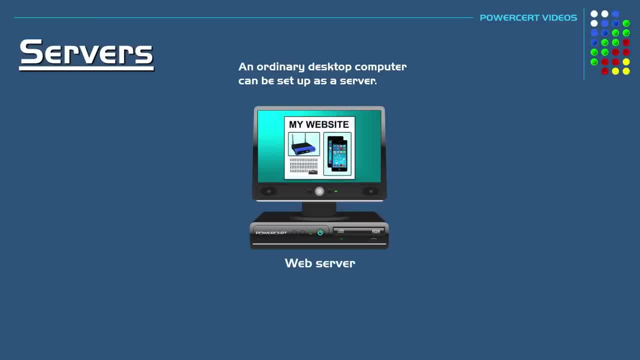 where you would install the website data on that computer and then the other computers can connect to it and retrieve the web page. However, desktop computers do have their limitations, because they are not designed to handle a large workload and they can't handle 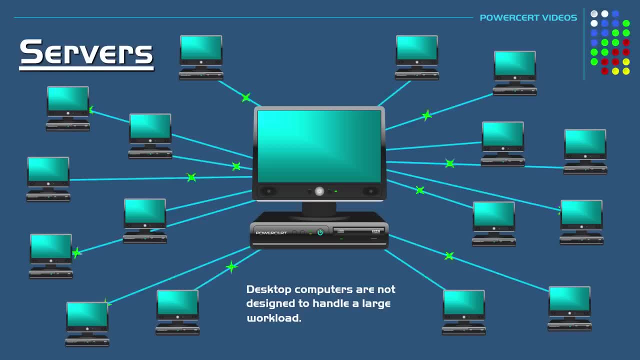 a lot of incoming connections from users, And this is not only because of their inferior hardware, but it's also because of software, Because desktop operating systems are only able to handle a limited amount of concurrent connections. Now servers need to be able to handle a lot of. 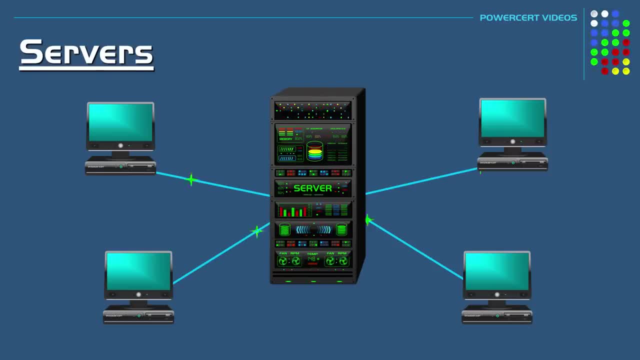 concurrent connections and they need to be up and running 24-7, because they are vital to an organization And if a server does go down, then that could jeopardize a business or an organization. So this is why servers need to be more reliable. They need to be built with robust hardware, that's. 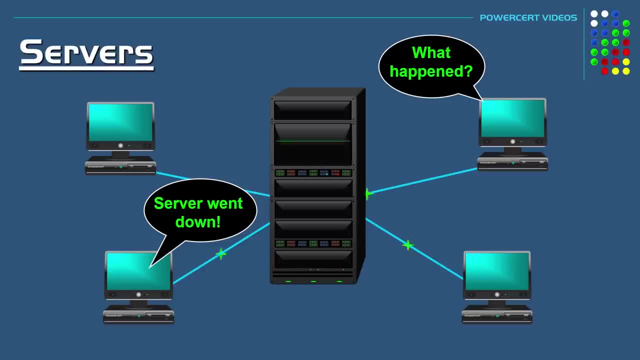 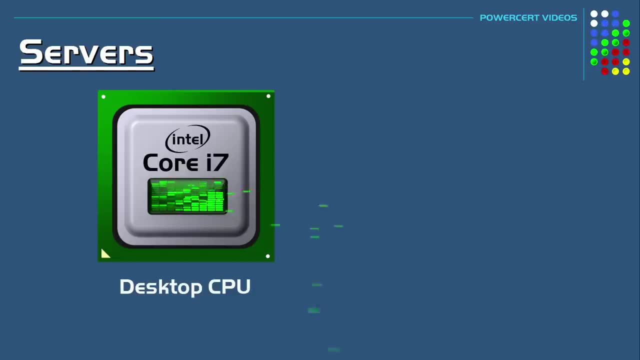 able to run non-stop with little to no downtime. So, for example, a desktop would use a processor that's designed, obviously, for desktops, such as the Intel Core 3.0, or the Intel Core 3.0.. Or a processor that's designed for core series processors And a server would use a processor. 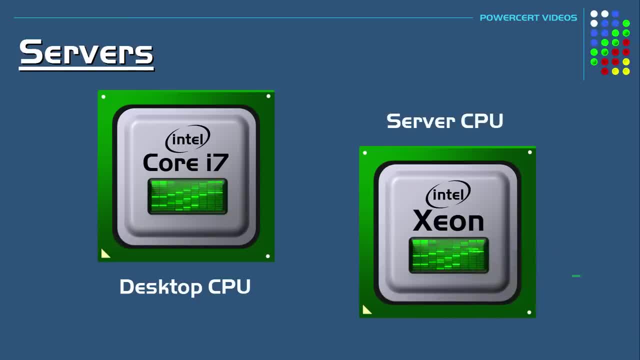 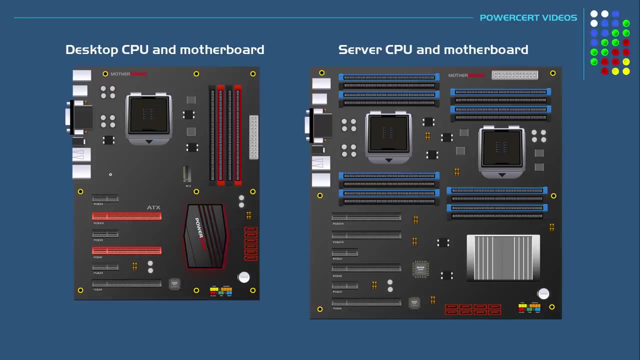 designed for servers such as the Intel Xeon processor. A server processor needs to be fast and have the ability to perform a lot of tasks simultaneously. Now, both of these processors are powerful, but there are some differences. So, for example, Xeon processors support a. 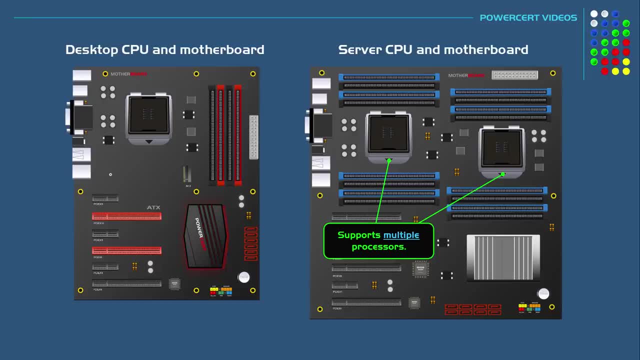 multi-processing environment, So they are designed to work with other processors, which means you can put two or more Xeon processors on a motherboard designed for servers, which is what a lot of servers need to handle a large workload, But desktop processors do not. 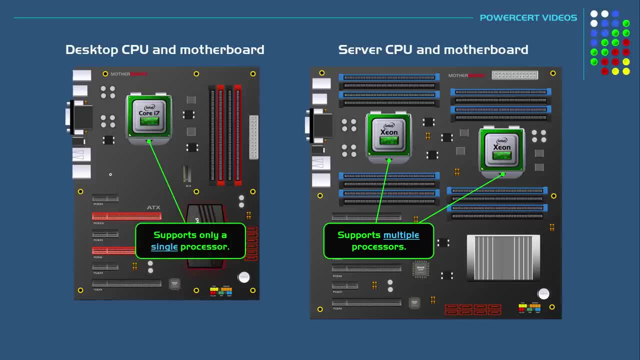 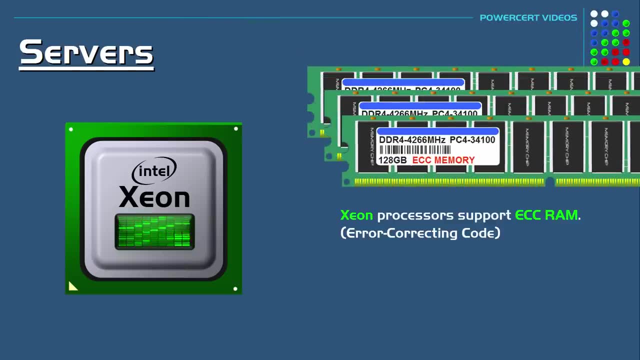 support this. They are only designed to work by themselves and not with other processors. And another difference is that Xeon processors support ECC RAM, which is Error Code Correcting Memory, And this type of memory is what's mainly used in servers Now. 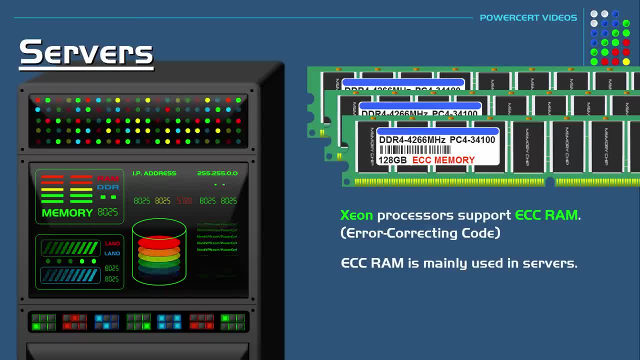 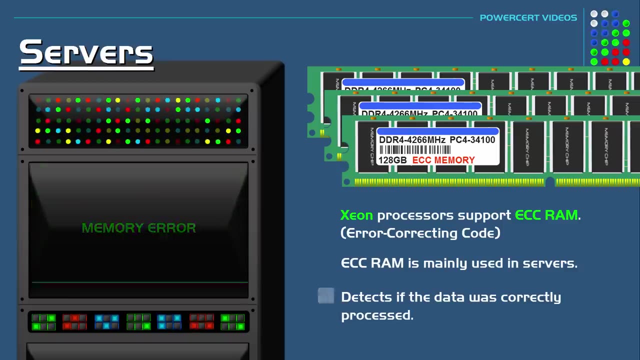 servers need to be up and running at all times and memory errors could bring down a server, And what ECC does is that it detects if the data was correctly processed by the RAM module and it makes a correction if it needs to to prevent memory errors. So, using ECC memory in 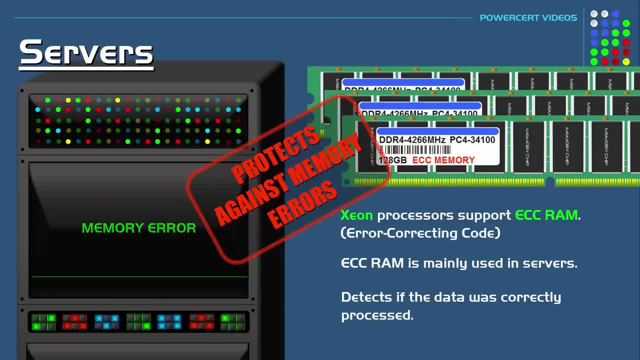 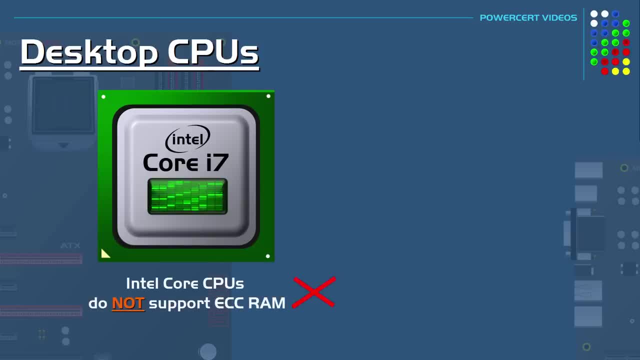 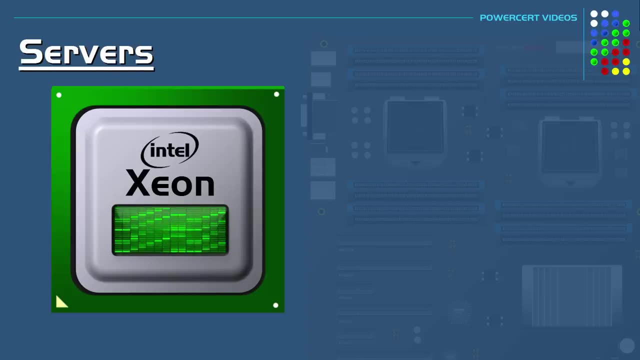 servers is just an extra precaution to guard against any errors, to prevent a server from shutting down. And Intel Core processors do not support ECC RAM, And that's why I'm here to talk. however, AMD processors do support it. ZM processors can also support a larger. 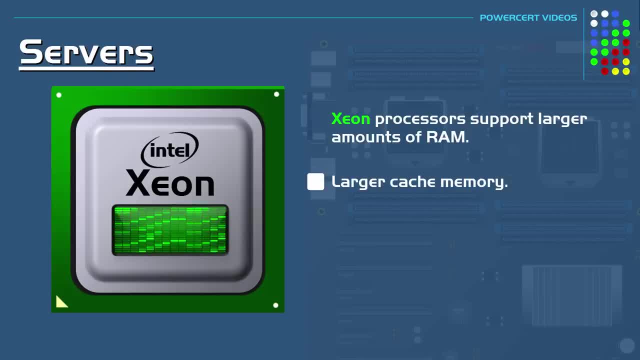 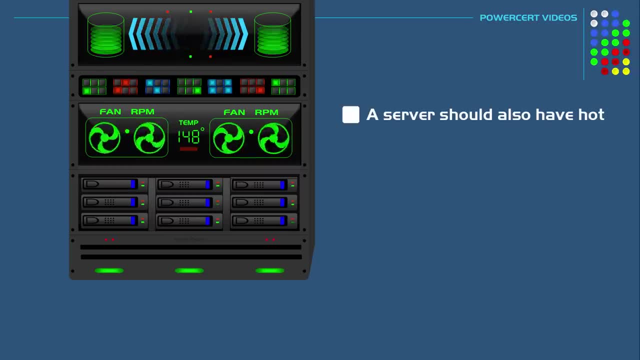 amount of RAM, they would have a larger cache memory and they would also have a higher core count than desktop processors. And a server should also have hot swappable hard drives in a RAID configuration, because if a hard drive were to fail, then no data loss would happen and the server would still be up. 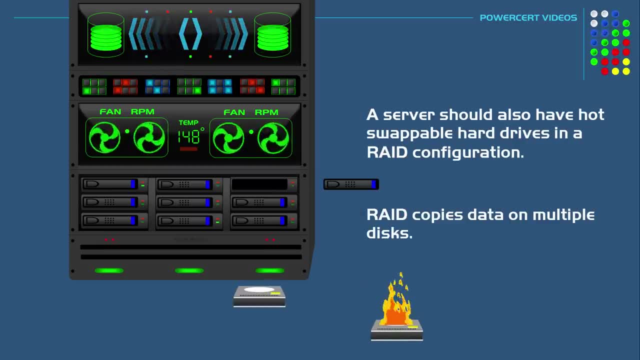 and running because of RAID. RAID is what copies the data on multiple disks, and if a hard drive were to fail, then it can be removed and replaced without shutting down the server, and then RAID would rebuild the data on the new hard drive automatically. 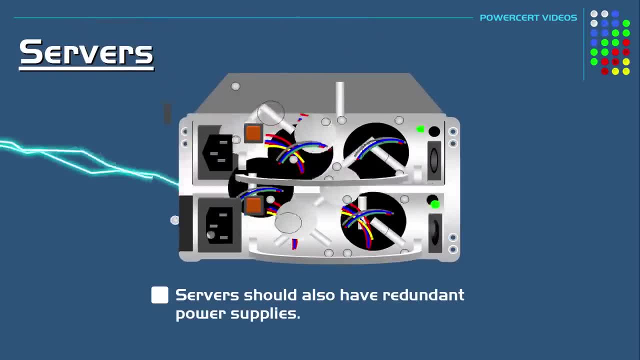 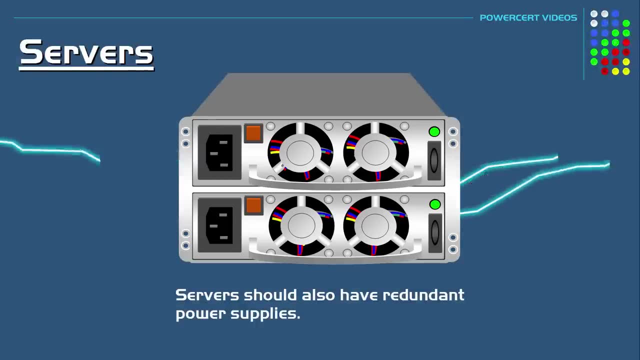 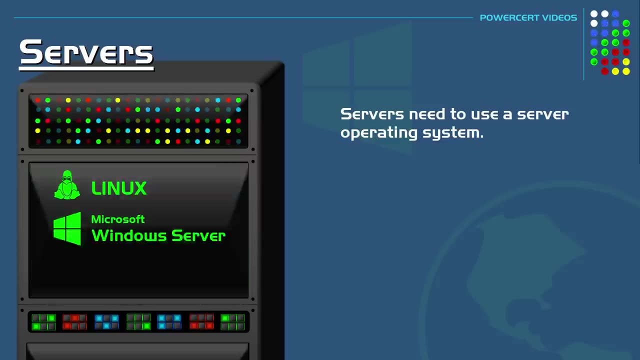 And a server should also have redundant power supplies to keep the server up and running in case of a power supply failure, And a server also needs to use a server operating system such as Linux, Windows Server, Mac OS Server and so on. Server operating systems are robust and stable. 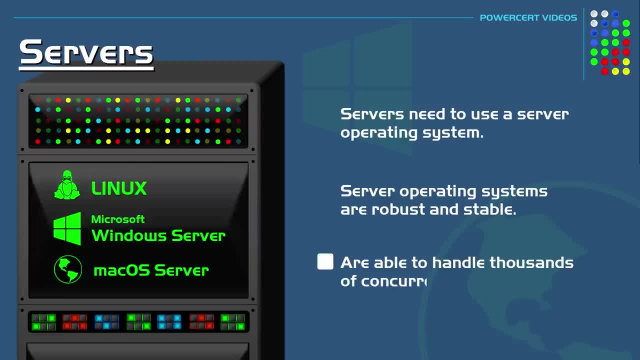 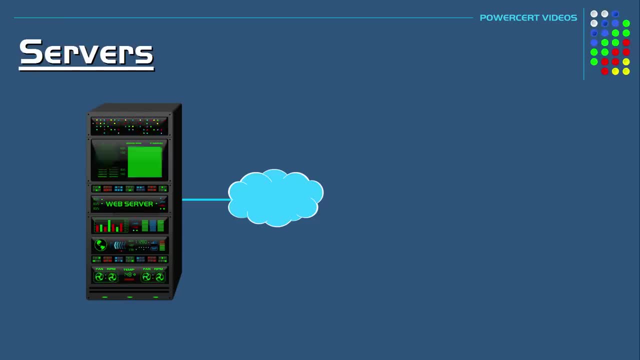 and they are designed to run non-stop and are able to handle thousands of concurrent connections. Now, there are many different types of servers, and when I mean types, I'm talking about the type of service that the server provides. So, for example, a web server. A web server is what hosts a website, So any 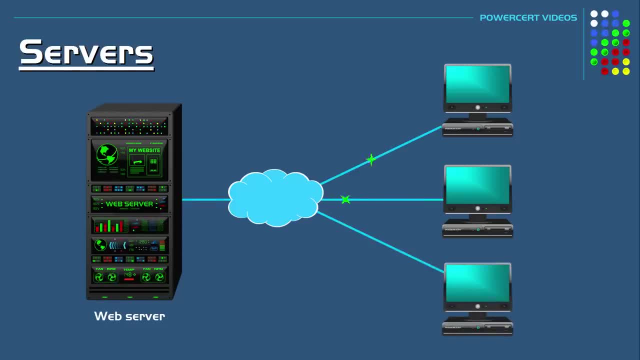 website that you go to with your web browser. you are connecting over the internet to that web server to pull up the website you want. The web server will contain all of the website's data, including the HTML code and graphics, and it'll also be running the web server software. Another type of server is an 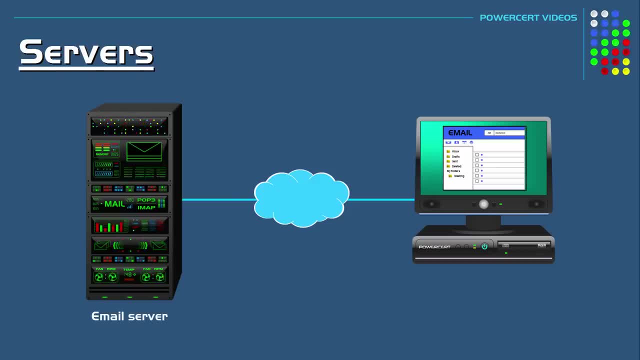 email server. An email server is what facilitates the sending and receiving of email, And you would access the email using your web browser, or you can use an email client such as Outlook or Thunderbird, using email protocols such as IMAP, POP and SMTP. And a database server is another.